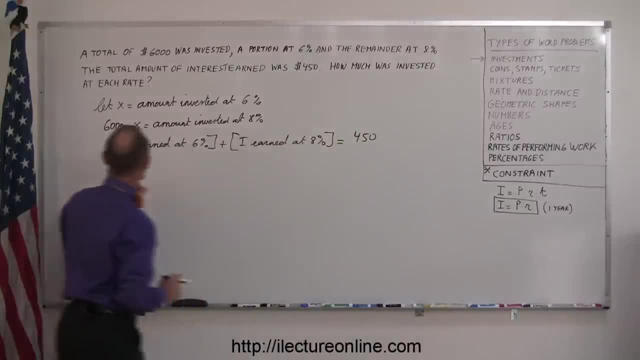 Coming back over here. it's the principal times the rate, So principal is x, the rate is 6%. So x times 6% is the amount that I earned at 6% Plus principal Principal times interest. so 6,000 minus x times 8%. 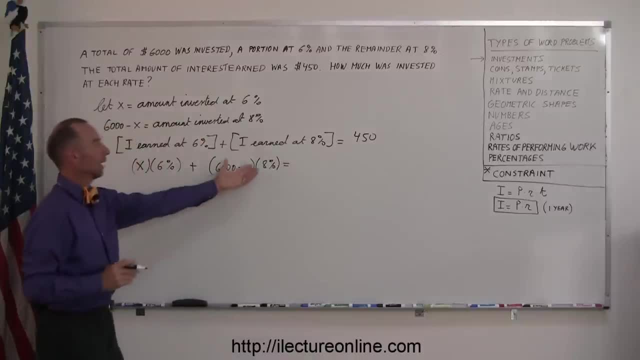 is the amount that I've earned at 8%, And added those two together, I should get $450 of earnings. Okay, now I'm ready to go ahead and solve this equation. First, I'm going to replace the 6% by its decimal equivalent. 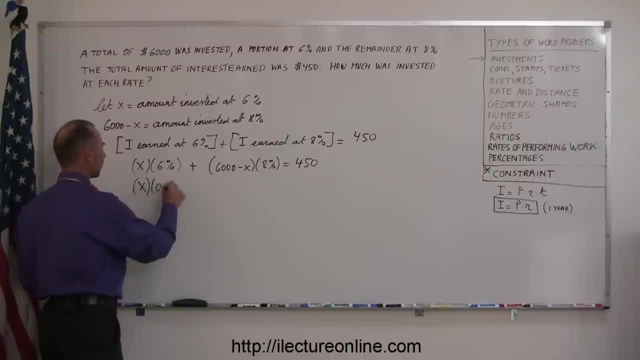 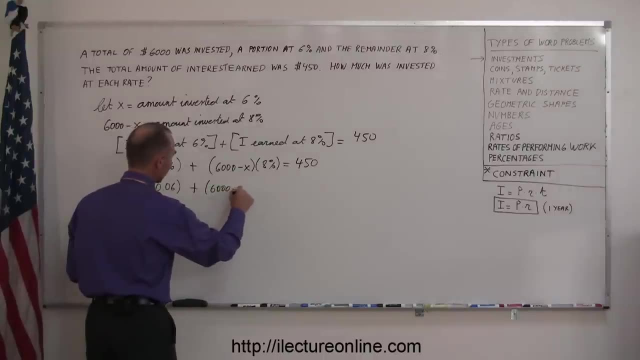 So x times 0.06.. That's the decimal equivalent. I'll say, oh my goodness, I do the same over here: 6,000 minus x times 0.08.. That's the decimal equivalent of 8%. 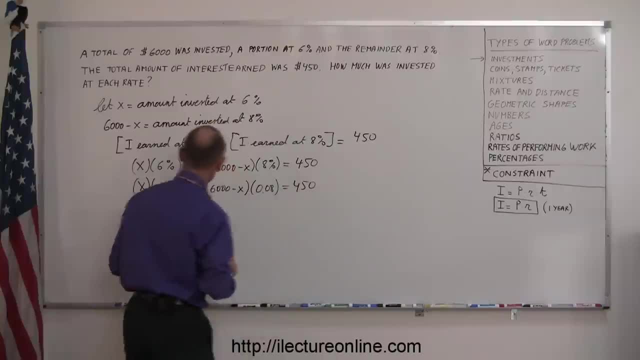 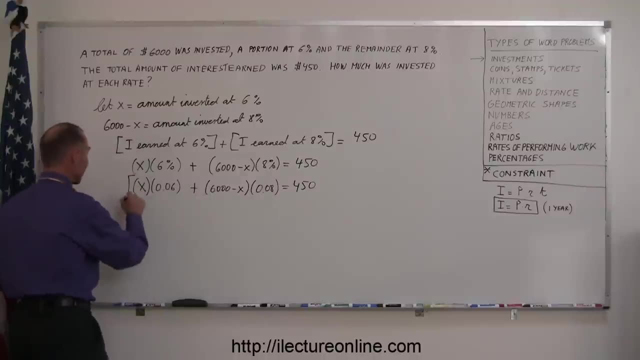 And that should add up to $450.. Now I'll go ahead and solve the problem. To do that, I want to first get rid of the decimal places. So to do that, I multiply both sides of the equation by 100.. Because I want to move the decimal place over two places. 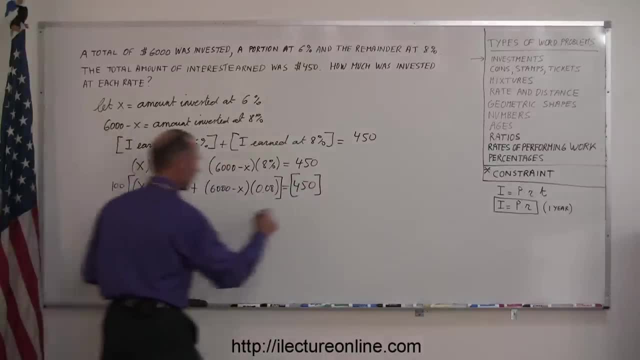 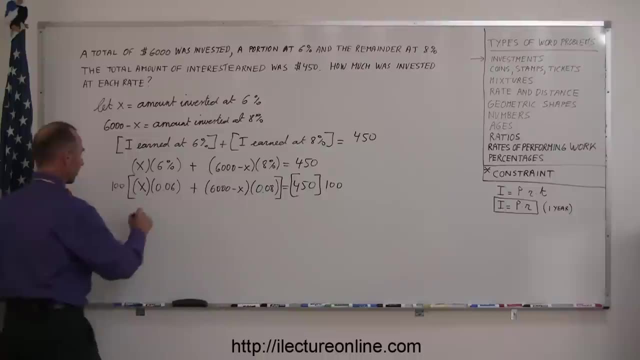 And, of course, whatever I do to the left side, I have to multiply both sides of the equation by 100.. So I'm going to multiply that to the right side as well. Okay, 100 times this- Well, 100 times 0.06 gives me 6.. 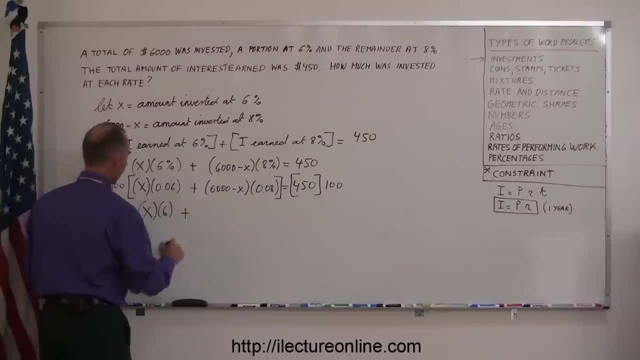 That's x times 6 plus 100 times this. When I multiply this, I get 8 instead of 0.08.. So this gives me 6,000 minus x times 8. And that equals 450 with two more zeros. 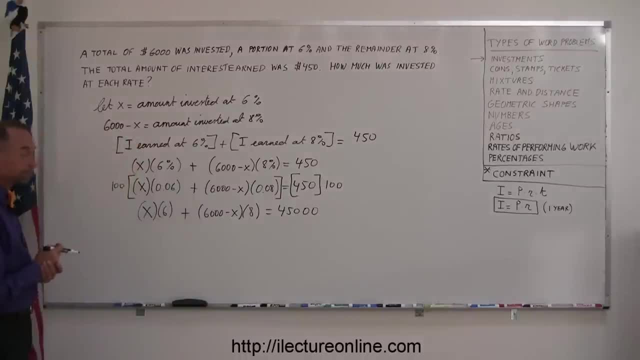 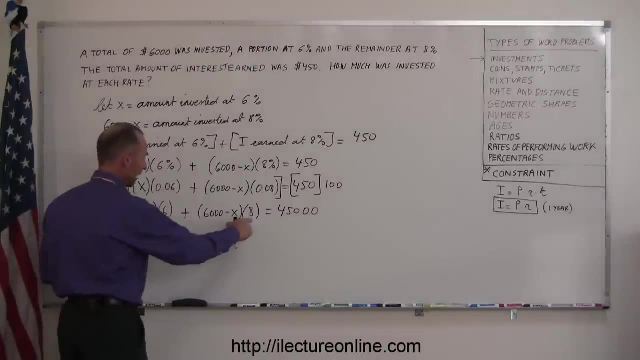 Because now I'm multiplying that times 100.. So I get 45,000.. Now we'll go ahead and get rid of parentheses And multiply everything together. So this is 6x plus 8 times 6,000 is 48,000.. 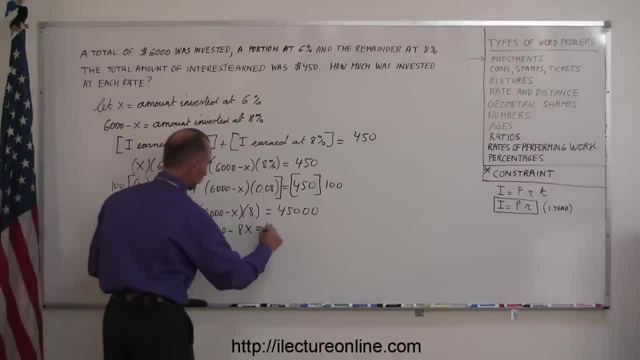 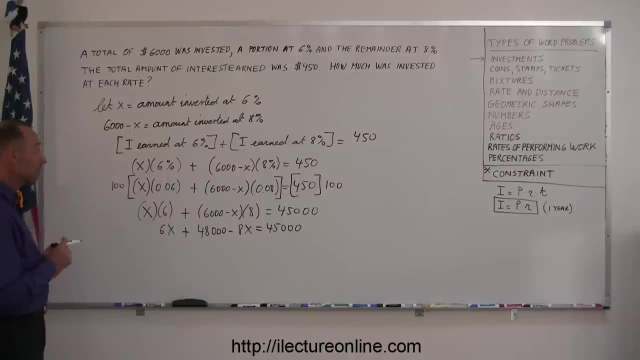 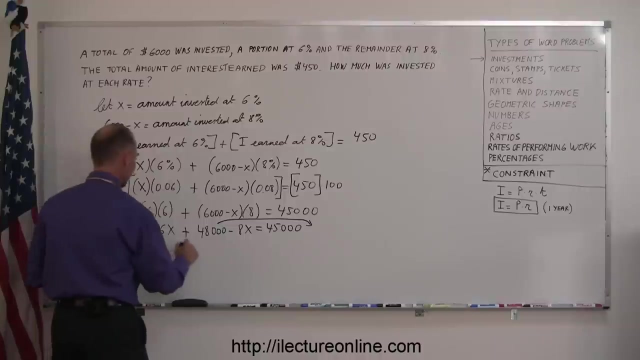 Minus 8 times x is 8x, And that equals 45,000.. All right. Next thing I need to do is move everything that's not associated with x to the right side. So move this to the right side, And so I end up with 6x minus 8x on the left side. 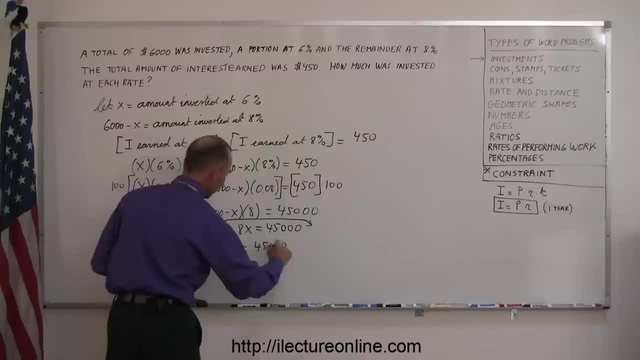 equals 45,000. And when I move the 48,000 to the right side I go across the equal sign. I have to change the sign So that becomes a minus 48,000.. Now I combine like terms. 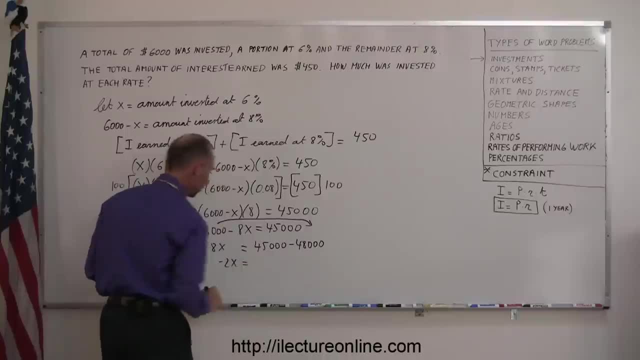 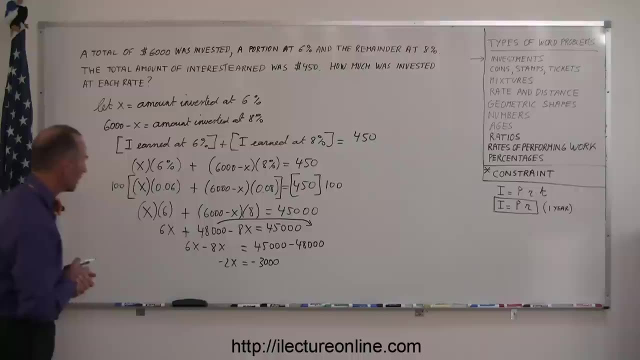 6x minus 8x is minus 2x Equals 45,000 minus 48,000 is minus 3,000.. And finally, I divide both sides of the equation by the numerical coefficient of x Or the negative 2.. 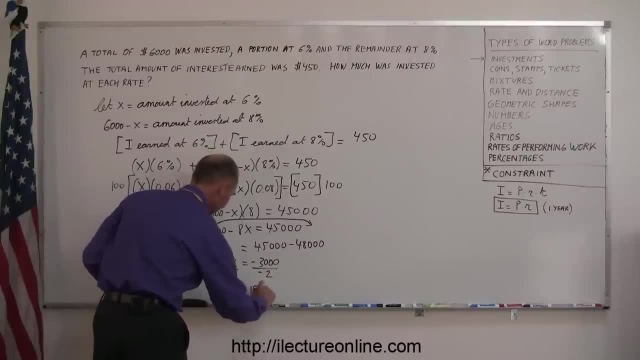 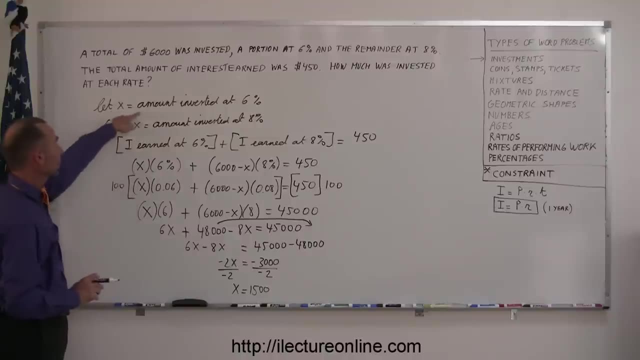 Negative 2.. So x equals 1,500.. All right, If that's correct, I can come back up here and say: okay, if x is the amount invested at 6%, that means I invested $1,500 at 6%. 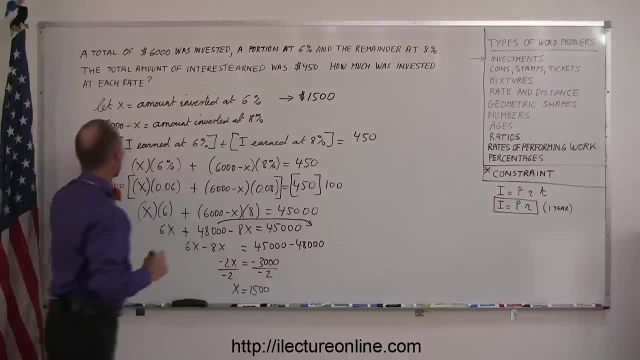 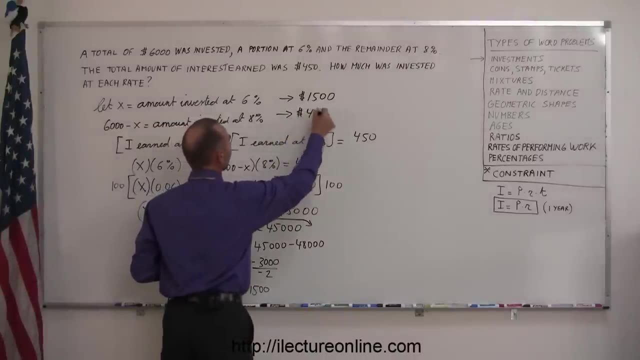 And 6,000 minus x, that's 6,000 minus 1,500.. That gives me 4,500.. So 4,500. At 8%. And now, just to make sure we didn't make any mistakes. 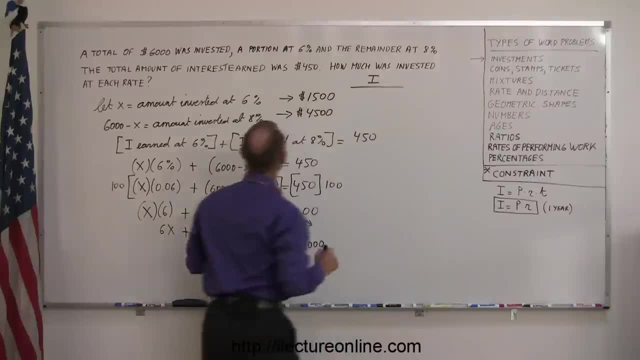 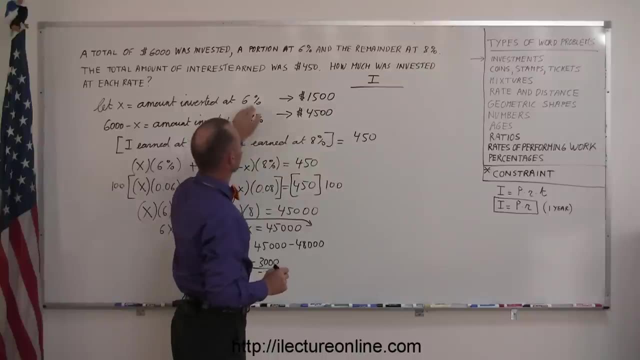 how much interest did we earn in each case? Okay, If I invest $1,500 at 6%, that will earn me $60, $90.. And if I invest 4,500 at 8%, that gives me 32,, 5, 36.. 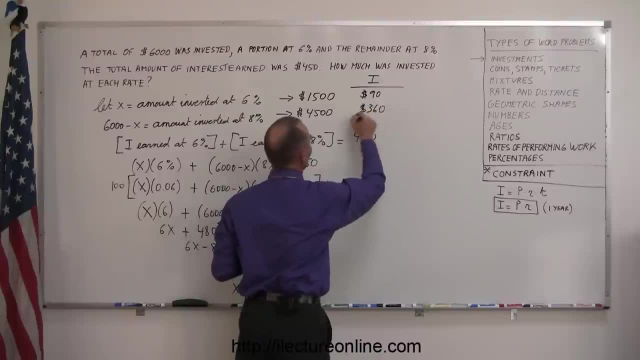 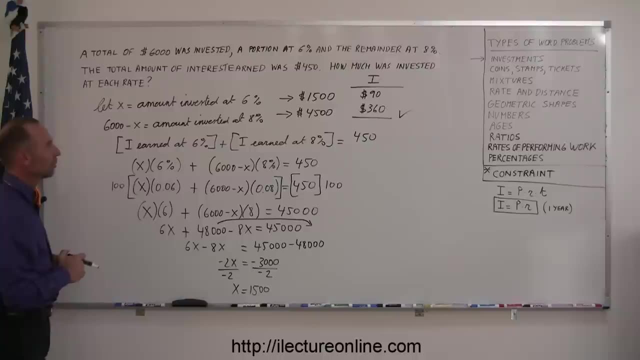 That gives me $3,360.. And does that add up to 450? It certainly does. So I did it correctly. All right, You always want to make sure that you do this correctly. Now, if you say: well, what did he do over here? 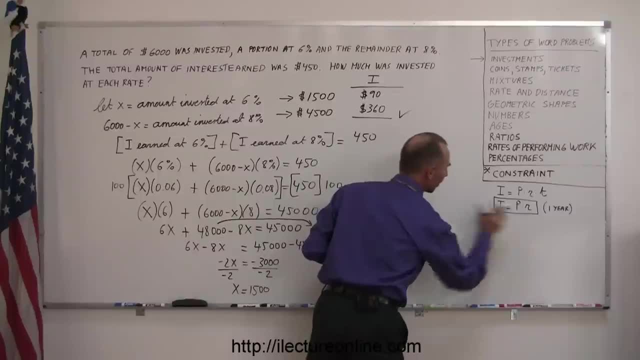 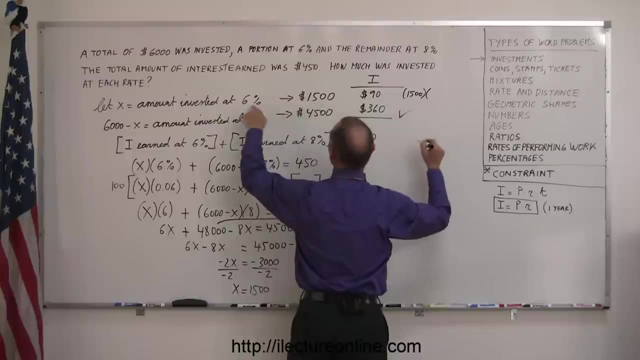 I didn't quite get that Well. what I quickly did is I applied this equation right here. I took the principal, So I said $1,500 times the 6%, which is 0.06.. When I multiply these two together I get 90.. 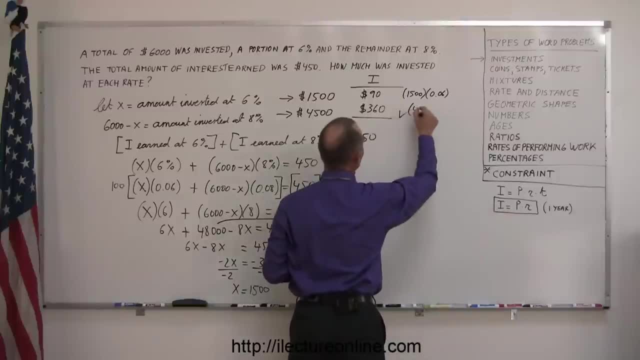 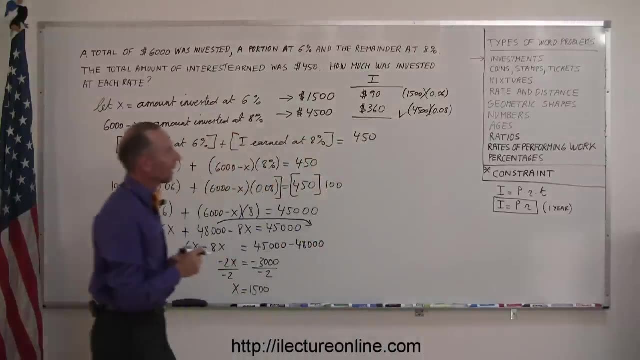 And over here I took principal times rate, So I took the 4,500.. I took the 4,500 times 0.08.. Quickly did that in my head and said ah, 360.. Together it adds up to 450.